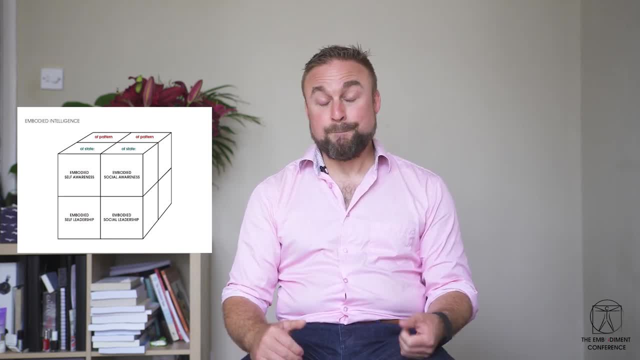 my state. I can go back and change my state. I can change my state. I can change what I can do in a moment. I can do it. I can move a little faster. I can move quickly. I can do a little faster. I can take a breath and change my state. I can do it more quickly. 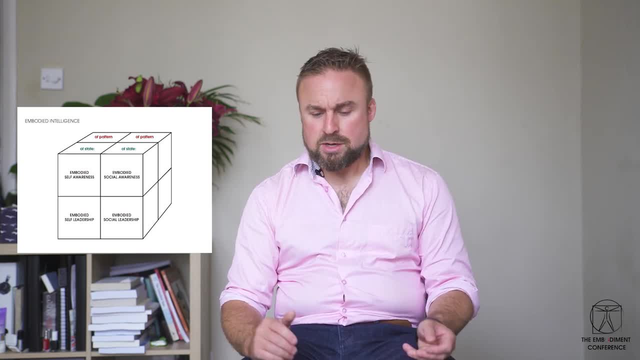 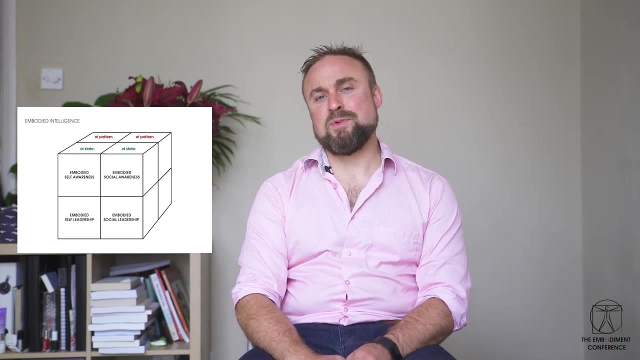 So that's how we develop our being, our embodiment in more a long-term sense, The intrapersonal side of things you'll see on the graphic, That's the left-hand side. On the right-hand side, some embodiment practices are very much about social awareness, So something 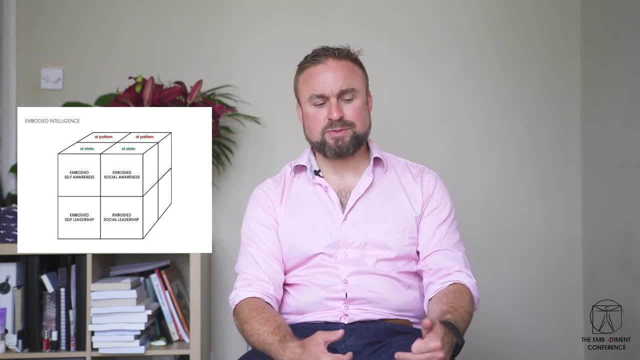 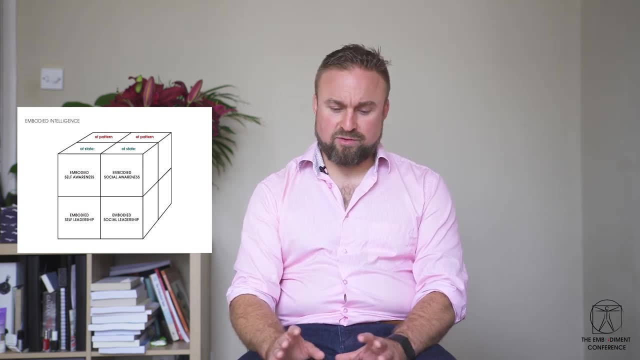 like circling, authentic relation. They're really looking at this Some kinds of partner dance. How is my partner, how is the group aware of the other, aware of the relationship? and again, that could be them, their state, how they are right now, or more like. 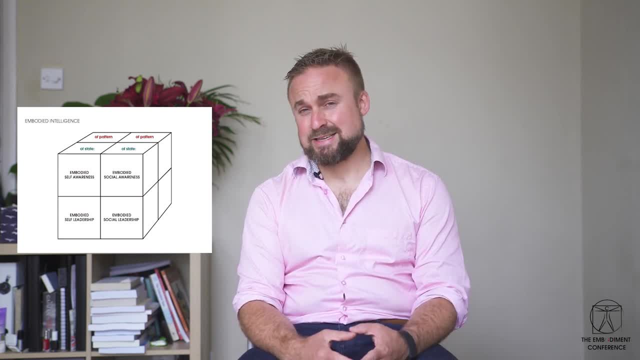 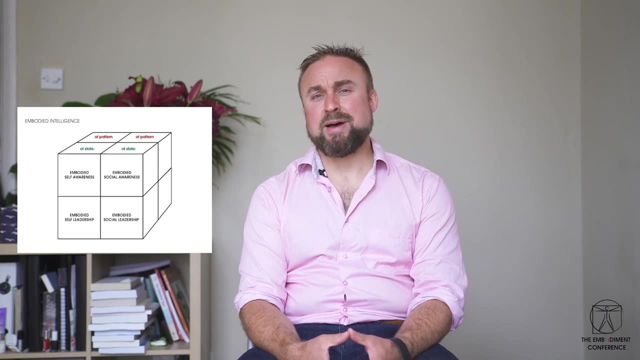 looking to observe, like body reading. they sometimes call that somatic assessments, looking at them more long term, so some teachers are more concerned with that. lastly, we have impact and influence, so it's: are you able to impact people? are you able to lead people to turn them on, to make them laugh, to calm? 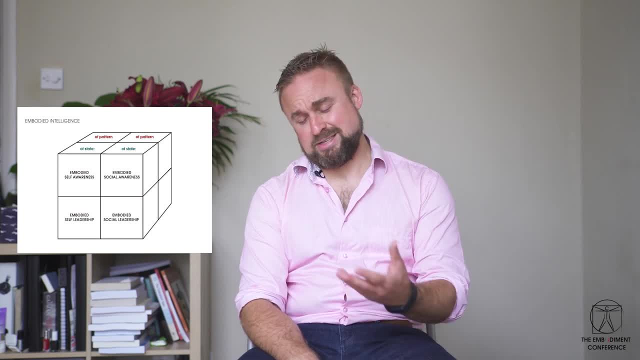 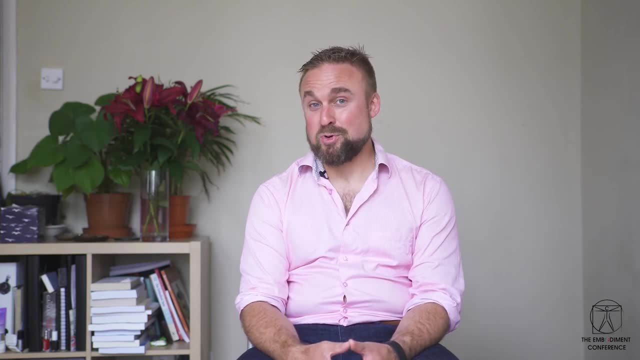 them down. whatever the impact you want is on their embodiment state trait would be like coaching someone to develop themself. look at my book if you want to go into much more detail about this model. you've got that free as a PDF if you registered for the conference. but yeah, looking at the embodied. 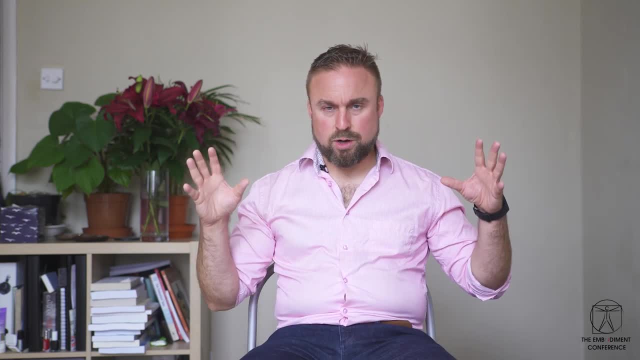 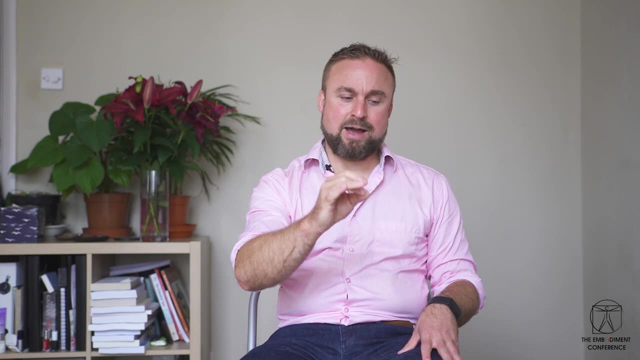 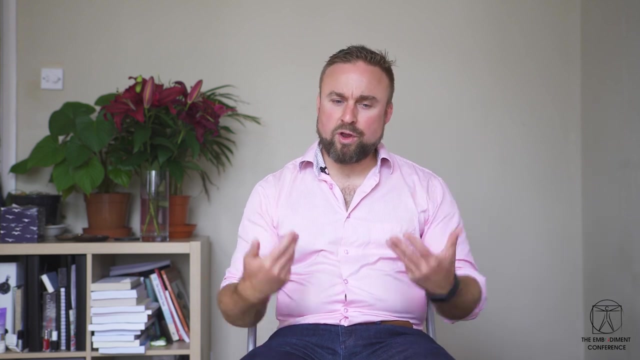 intelligence gives a really clear framework. what I like about it is that it's um, it's not esoteric, it's you can look at how you, what skills you have, what skills aren't so good, what practices develop them. so it's a really nice model to orientate. to the conference towards.